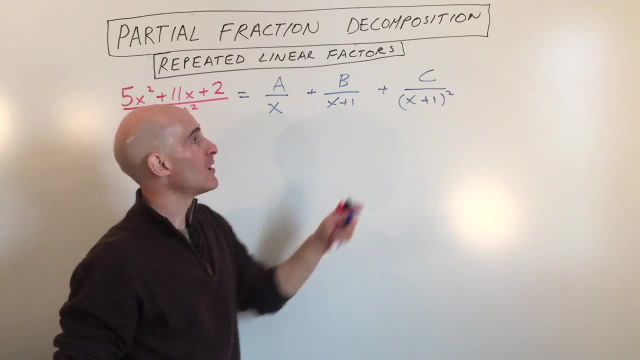 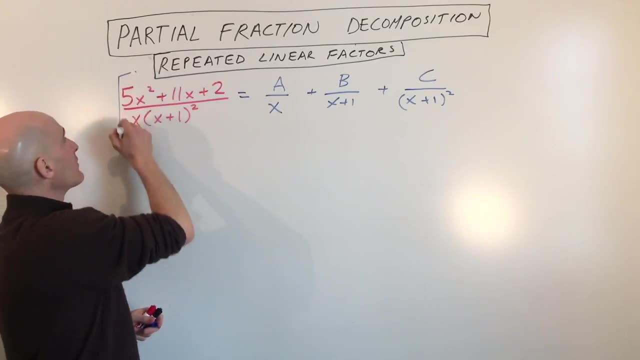 factor. This is a linear factor, so this is just going to be one degree lower. Okay, so now all we have to do is we just have to clear the denominators and solve this equation. So we're going to multiply the left and the right sides, the entire equation, by the common denominator. This is the common denominator here. x times x plus 1 squared. So when we multiply each of these fractions by that quantity, we clear the denominators, and we're left with 5x squared plus 11x plus 2. Here, the 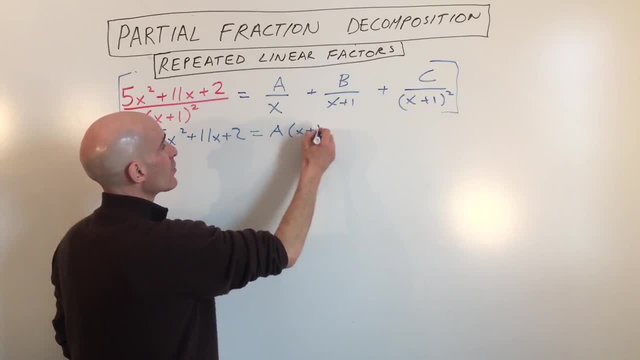 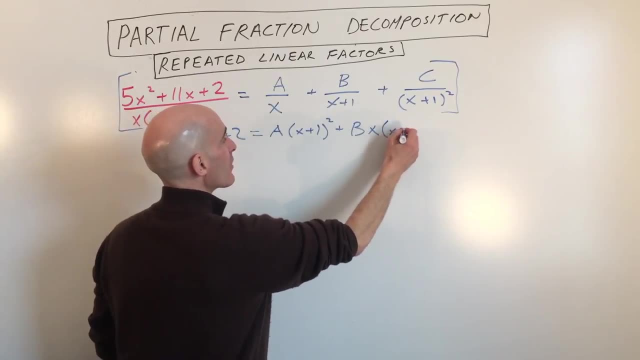 x's are going to cancel out. We're going to have a times x plus 1 squared, plus, here we're going to have b times x times another x plus 1, because one of the x plus 1's is going to cancel. And then the third one, when we multiply, we're going to be left with c. 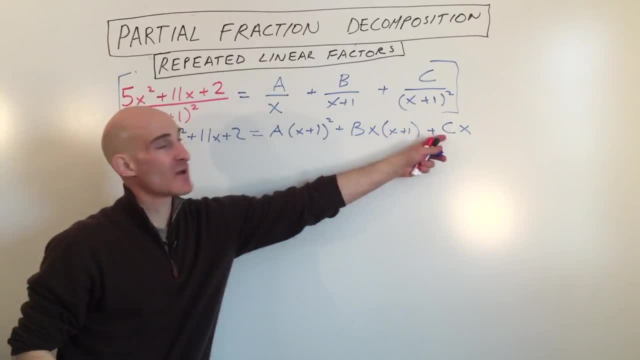 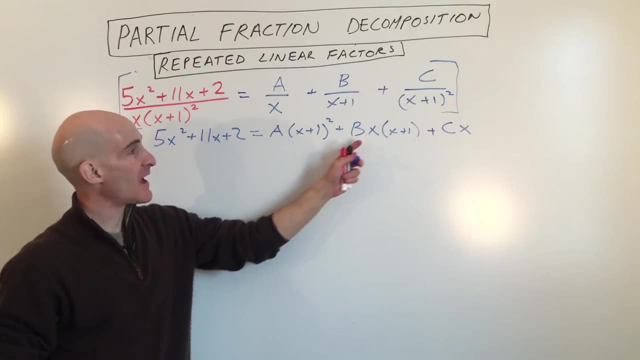 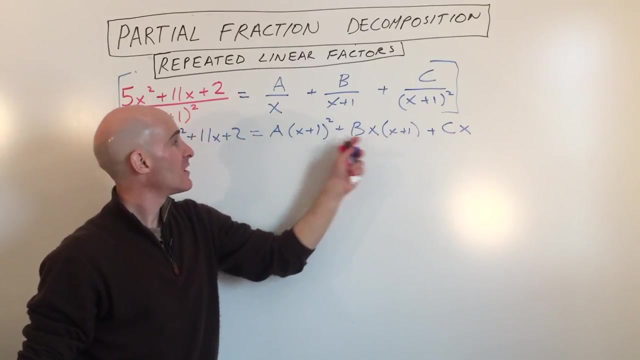 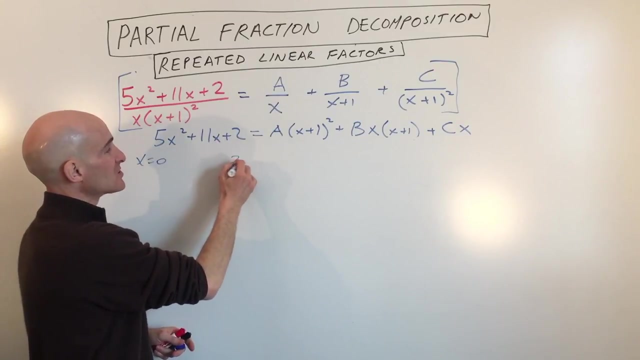 c times x. So we've cleared the denominators by multiplying through by this common denominator. Okay, so what do we need to do now? Well, we're going to be strategic, and we're going to say let's let x equals 0, because if we do that, 0 times anything is 0. That's going to cancel out these two groups, and we can solve for a. So let's let x equals 0. x equals 0. So that's going to make this 0 plus 0 plus 2 equals 0 plus 1 is 1. 1 squared is 1. That's going to be a. 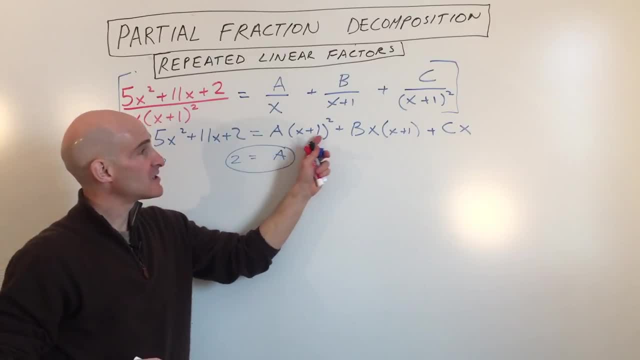 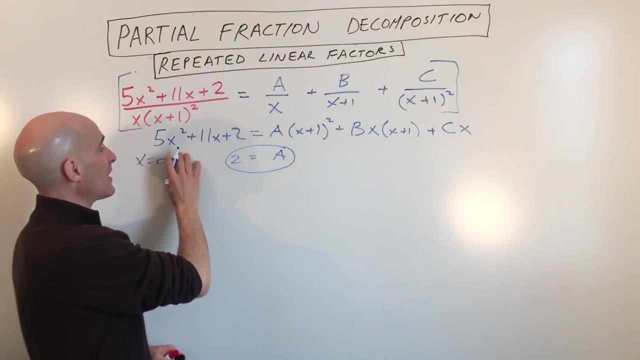 Let's be strategic again. Let's set x equal to negative 1. That'll cancel out this term and this term. We'll be able to solve for c. Okay, so let's do that. So we put x equals negative 1. We get negative 1 squared is 1 times 5 is 5. Okay, plus negative 11 is negative 6, plus 2 is negative 4. Okay, negative 1 plus 1, that's going to make this 0. That's going to make this 0. That's going to make this negative c. So you can see that it's 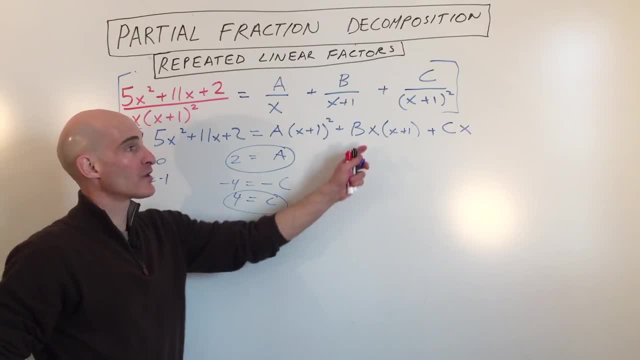 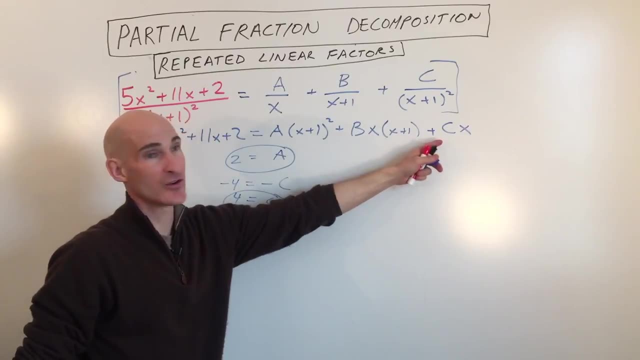 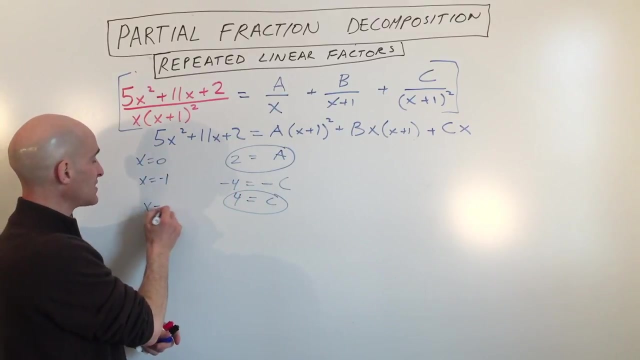 c equals positive 4. Now all we're left to solve for is b. Well, there's we can't cancel anything out by being strategic by setting x to a certain value to cancel out some of the other terms. So why don't we just let x equal positive 1. Okay, so we're going to say x equals 1. We put in 1 here, we get 11 plus 5 is 16 plus 2 is 18. a we already know 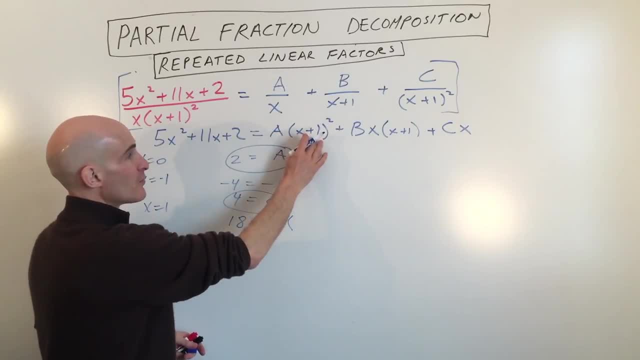 is 2, and we're putting 1 in for x. That's 1 plus 1. It's 2. 2 squared is 2. So we're going to put x equal 1. And we're going to put 1 in for x. So that's 1 plus 1. That's It's 2, 2 squared is 4. 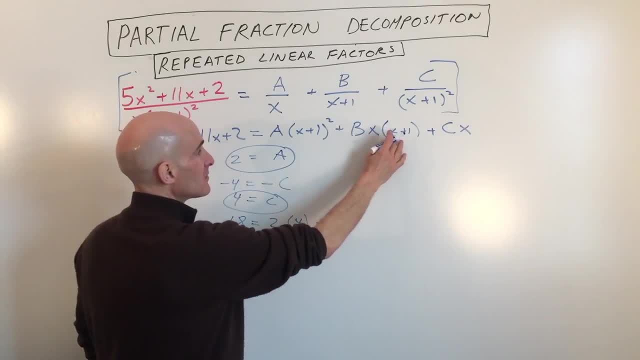 Okay, b we don't know, times 1, times 1 plus 1 is 2, so that's going to be b times 2, plus c we know is 4, so that's 4 times 1, which is 4. 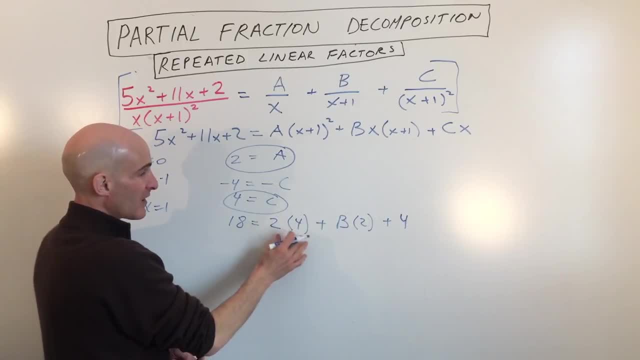 Now we can solve the equation for b. So what do we have here? We've got 8 plus 4 is 12, subtract the 12, that's going to give you 6, equals 2b, so by dividing we get b equals 3. 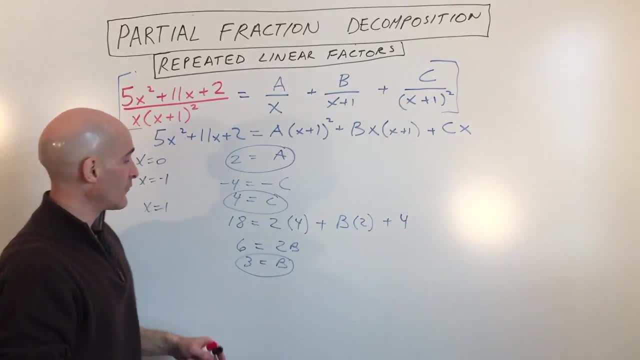 Now we know a, b, and c, and if we go ahead and put these back in, you can see that these would be your original fractions before you combine them together to get this fraction here. 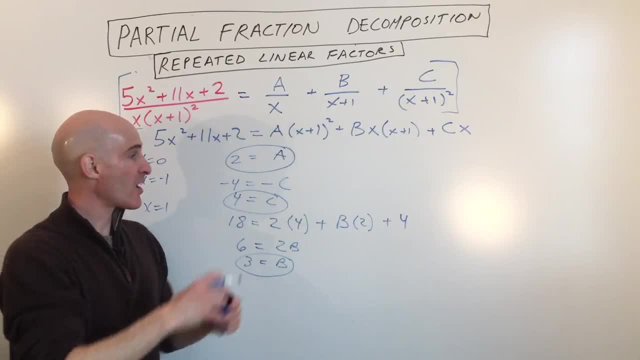 So we decompose it, we broke it down into the original fractions prior to adding them together. 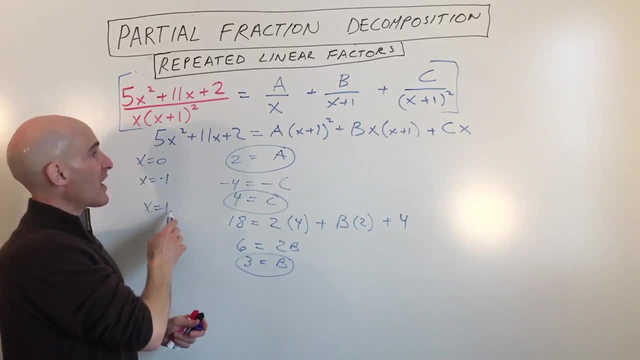 So again, this is a good technique, you know, by picking certain values for x to cancel out some of the terms, but sometimes you'll get to the point where, you know, you'll have to just pick a value like we did here at the end, we substituted x equals 1 in, and we used the other values that we solved for already. 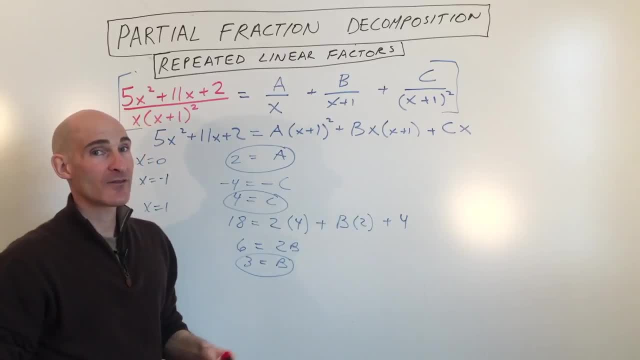 Now if we had a couple other variables left over, we'd have to solve a system, and I can show you how that works in some of the other videos. So I'll see you in the next video. 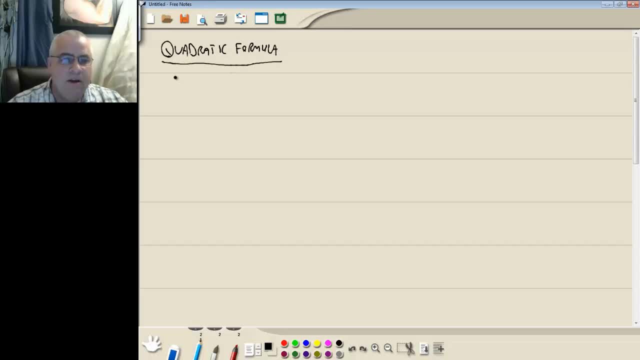 With our quadratic formula, the problem has to be of this form. ax squared plus bx plus c equals zero. Quadratic. You can have any variable. It doesn't have to be x's. a, b, and c represent numbers. Typically integers, but they don't have to be integers. Now if you get it in that form, the quadratic formula says your answer is going to be x is equal to negative b plus or minus square root of b squared minus 4ac all over 2a.